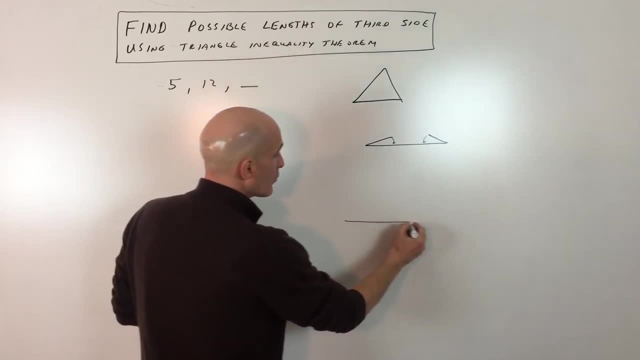 twelve. let's see if we can just sketch it out, just to give us a visual way of appreciating this. So here's twelve and let's just say that here's five, right, So the third side could be like that, right? But you see this point right here, This is like a hinge, okay. 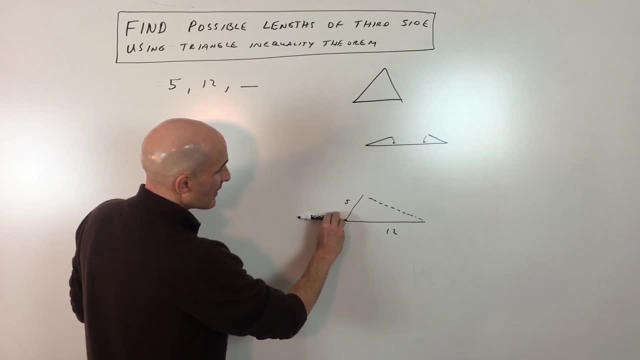 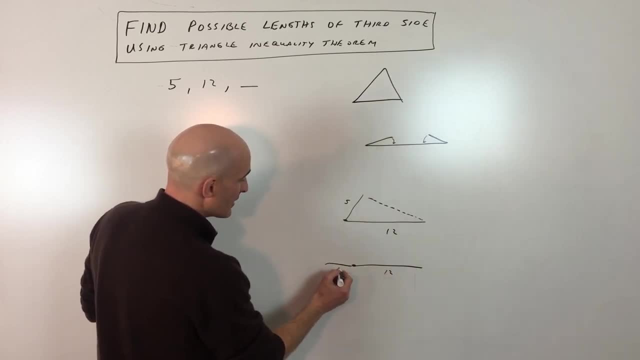 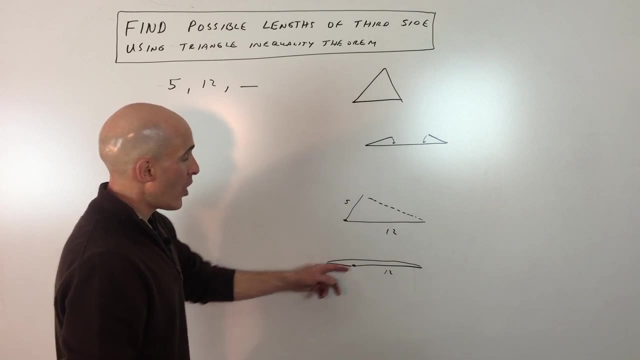 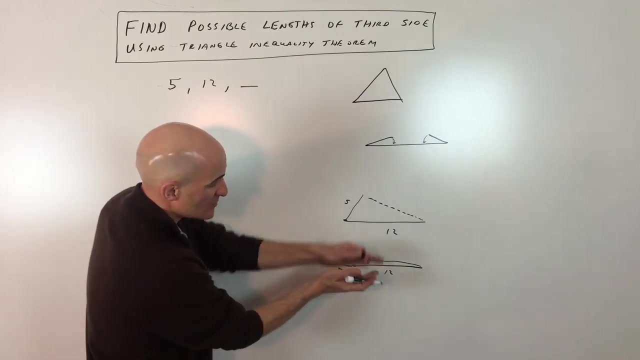 this is twelve and this is like five right here, and then the third side would have to span that distance like so right. So the longest this side here could be would be up to seventeen, not including seventeen, because if it was equal to seventeen, this would actually. 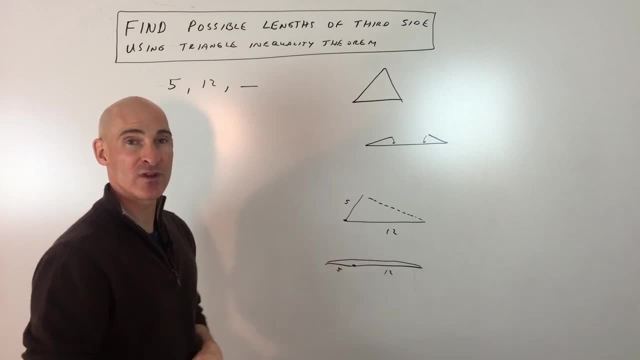 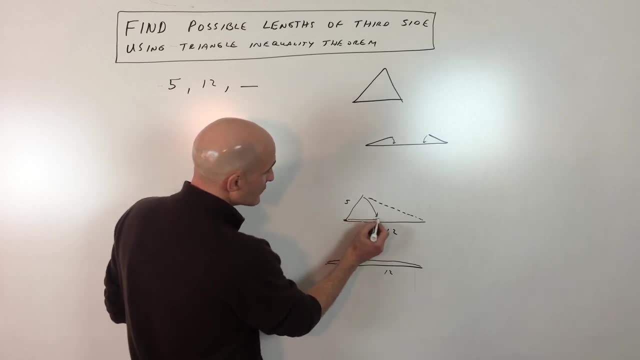 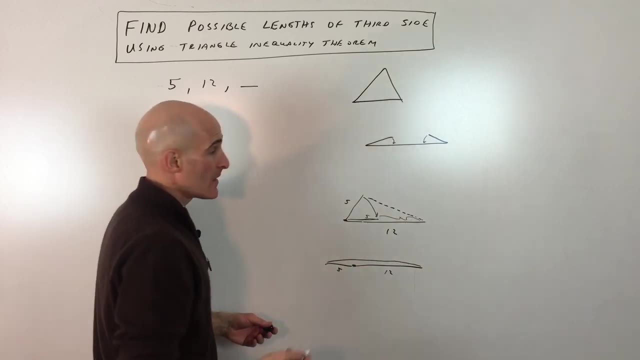 that if we were to take this side here and rotate it down like this, so that five is like right here now, it only has to span this distance from here to here, which is only going to be seven units. So essentially, if you think about it as a hinge, okay, the most. 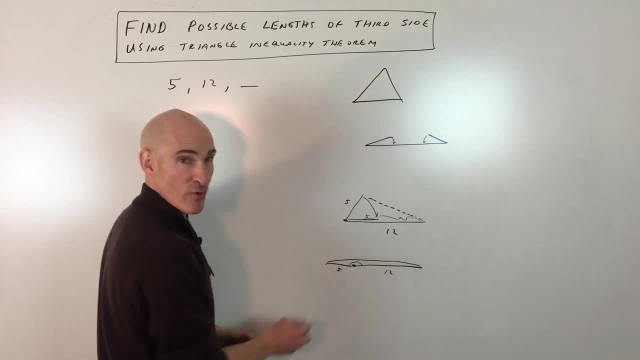 extreme example is when you make it like a hundred and seventy nine point nine degree angle, or you make it like a zero point one degree angle. right, It's either folding this way or it's folding like that. So, essentially what we have here for this third side, we'll 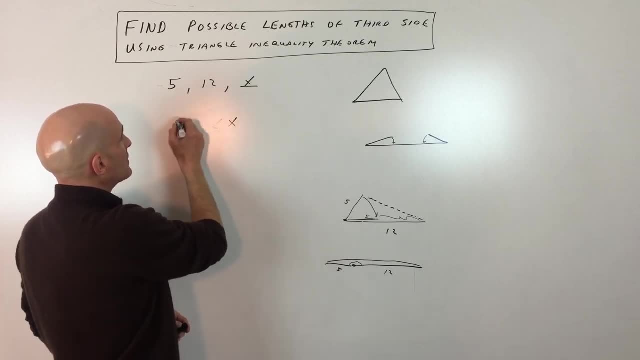 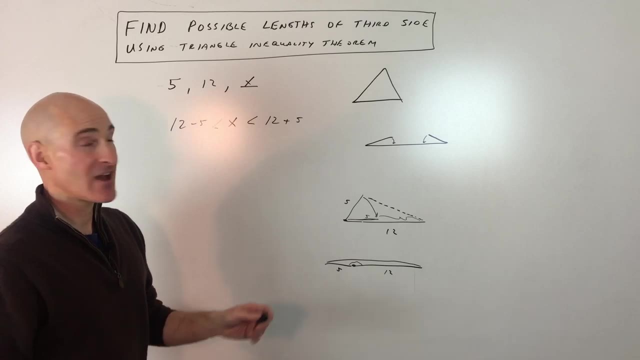 just call it x. it has to be greater than 12 minus 5 and less than 12 plus 5. so that's the shortcut. if you want to just get down to it, just a simple way of doing this: you can write it as a compound. 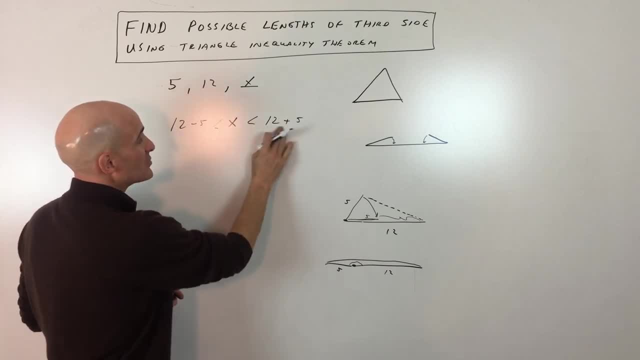 inequality and it's going to be somewhere in between the sum of the two sides and the difference of the two sides. so if we simplify, you can see x is greater than 7 and less than 17, not equal to, because otherwise then it's going to collapse on down flat. so that's how you would use a triangle. 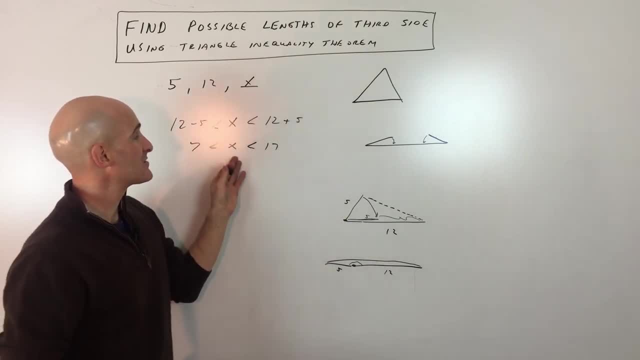 inequality theorem. to solve for the possible lengths of the third side again, the shortcut is just to add and subtract the two side lengths and that'll give you an interval of the possible lengths of the third side. so i hope this helped clear that up for you. subscribe to the channel.